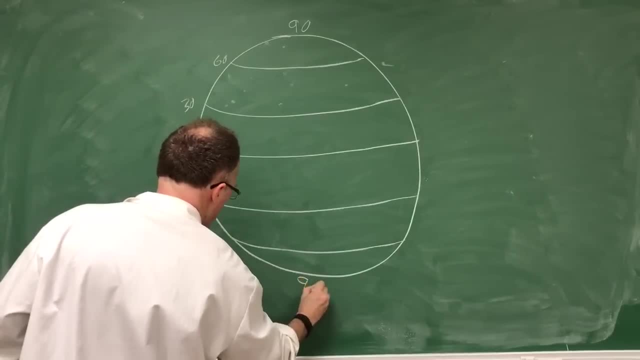 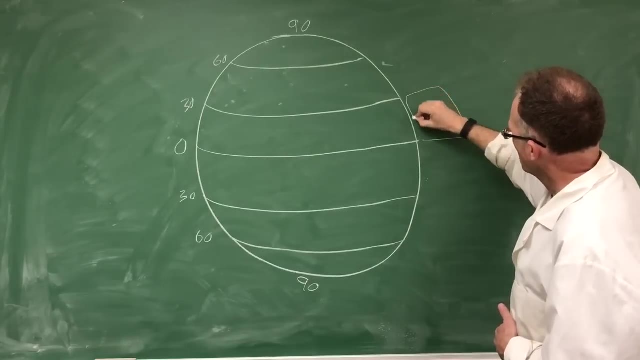 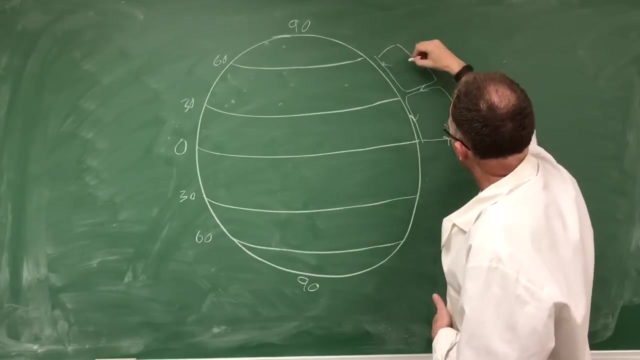 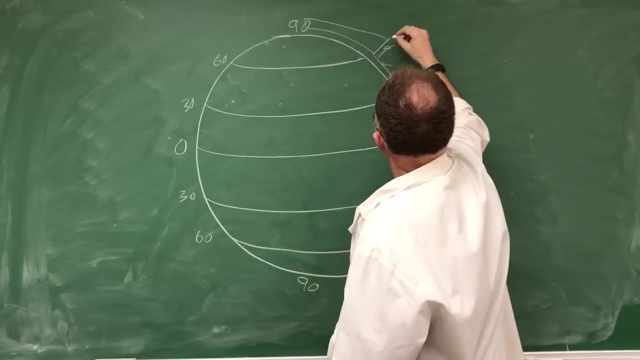 the southern hemisphere. Okay, you should be able to draw this from heart by heart. right, Air rises at the equator, spreads out, comes down here. Right, this is the Hadley cell, This is the Faro cell And this is the polar cell. so 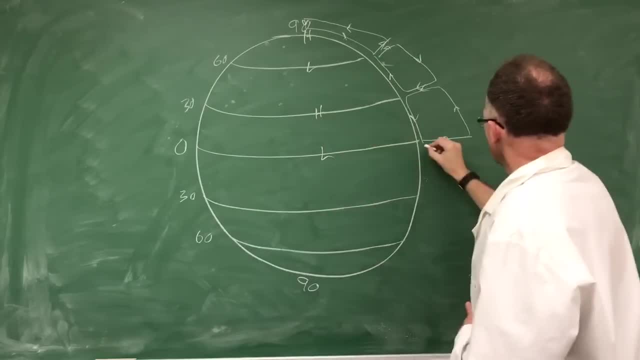 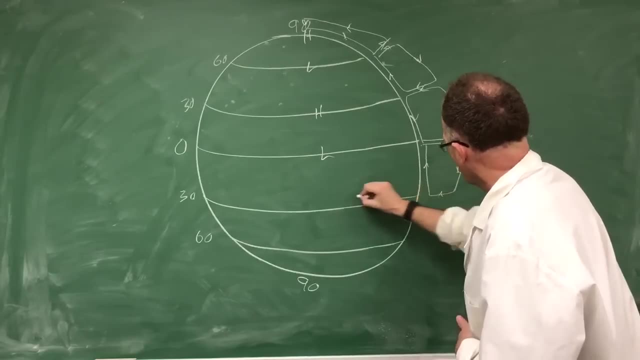 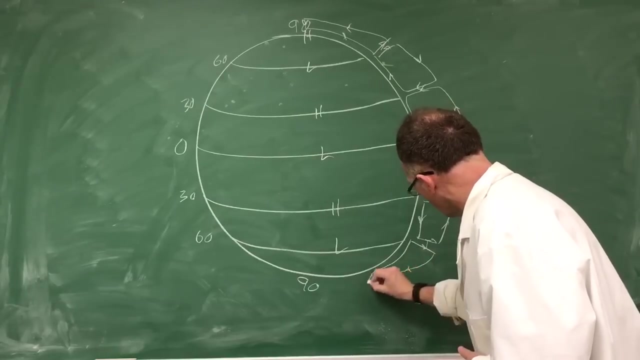 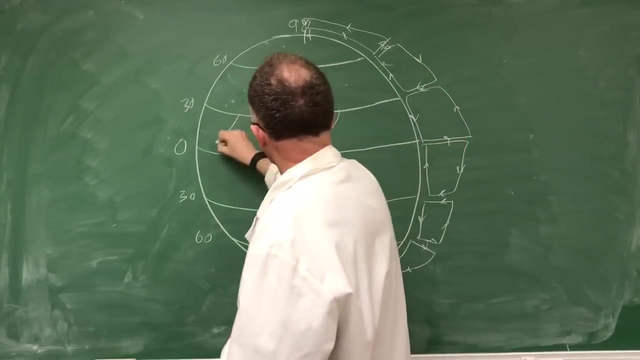 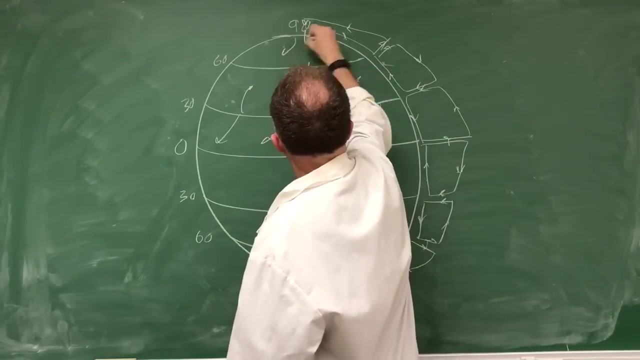 there's the high pressure, low pressure, high pressure, low pressure. Same thing in the southern hemisphere. Okay, high pressure, Low pressure, high pressure. So this is the equator: things turn to the right right, So we get this right. Northern hemisphere: things go to the right Right, so we get the. 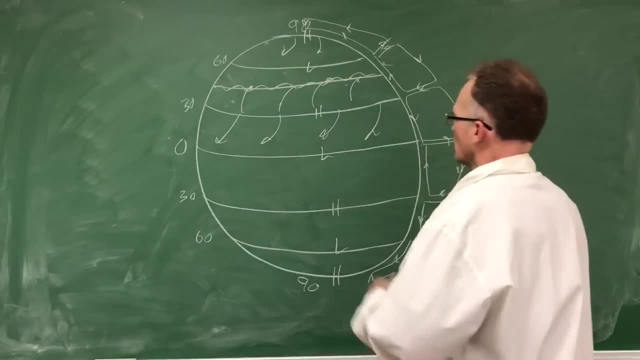 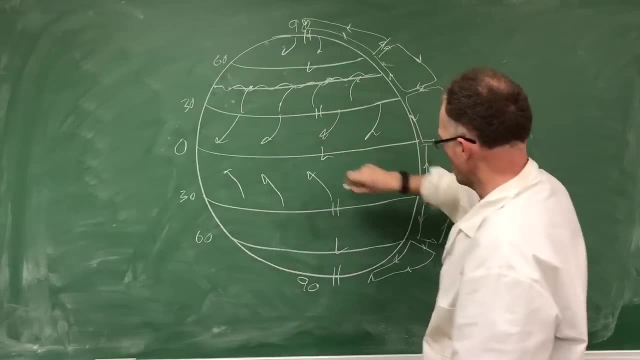 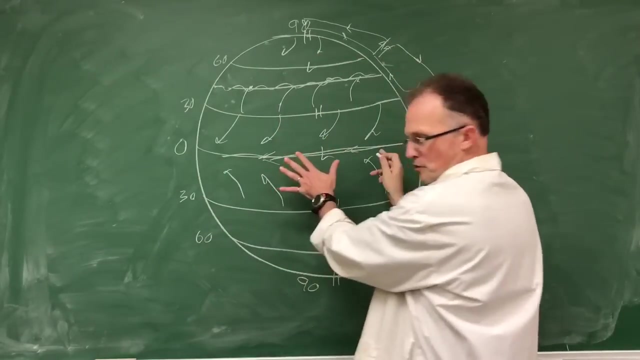 jet stream circling the Earth here. Okay, so same thing down here. things go to the left in the southern hemisphere from high to always, from high to low, but it deflects to the left in the southern. That gives us the trade winds here. So this gives us Walker circulation. It pushes the cold water away. 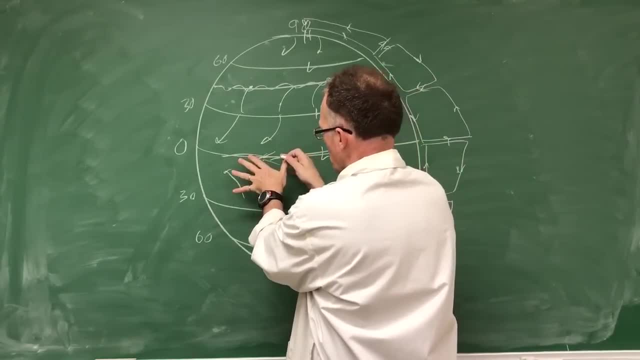 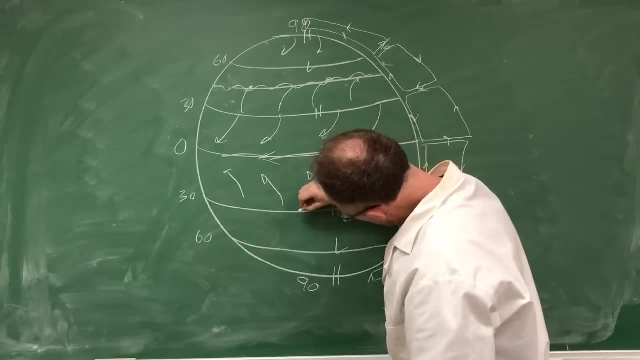 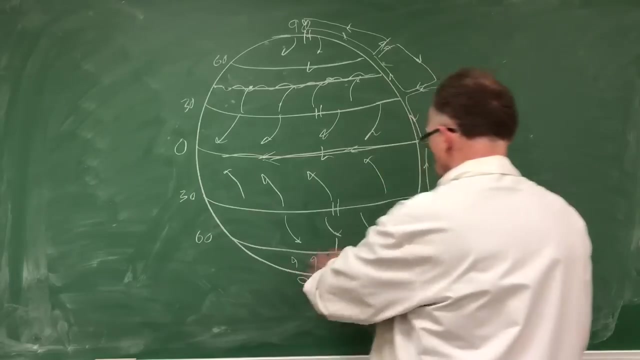 from South America towards the Indonesian archipelago. That water builds up. Eventually, the Walker fails, the water sloshes across, causing an El Nino. High to low deflection to the left. Okay, high to low, deflection to the left, So you can get different wind. 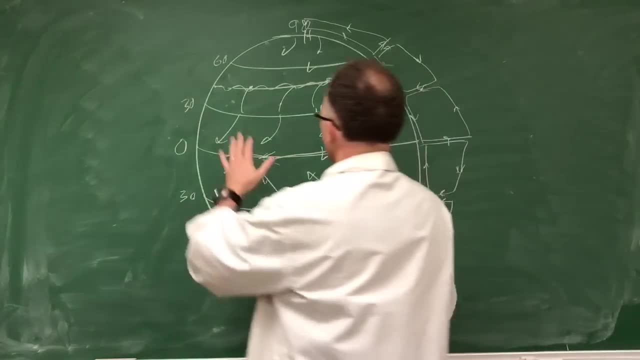 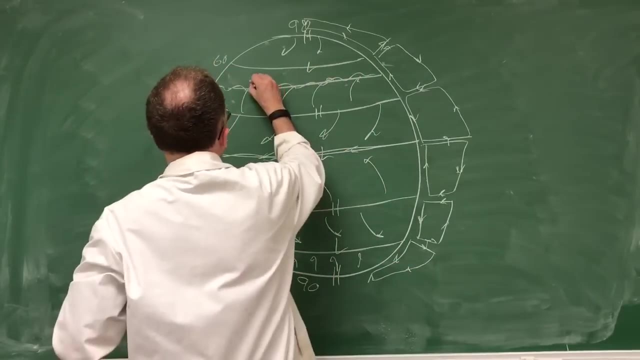 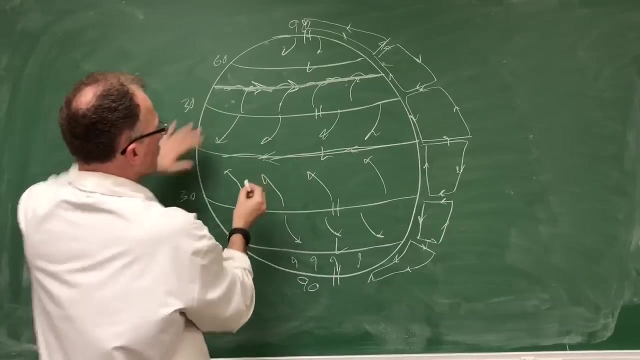 patterns and establish things. Okay so the jet streams are mostly zonal, going from west to east around the planet. Okay, so they're moving this way. you know they're moving this way. Okay, there's one over here. This is about 45 degrees north, Ottawa, Southern. 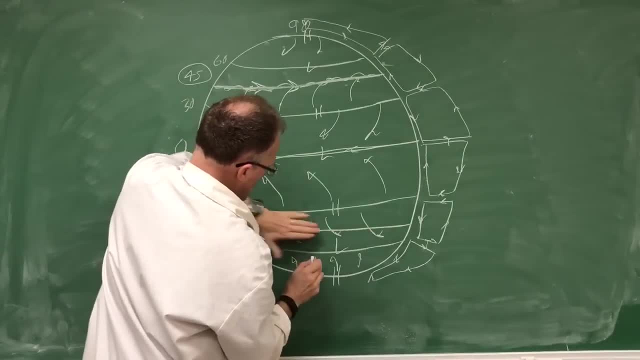 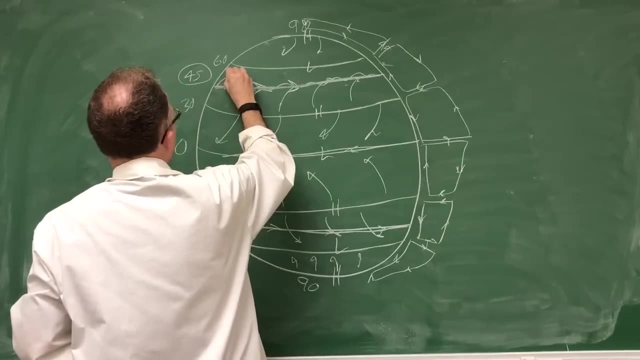 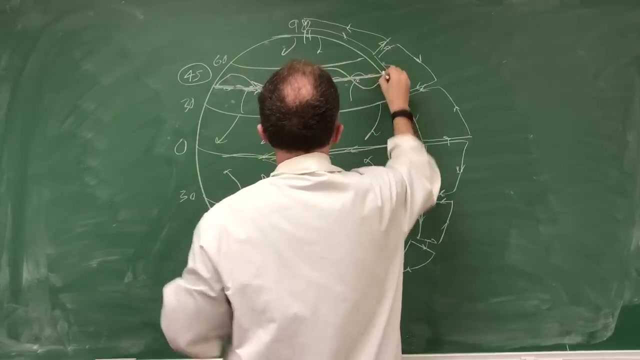 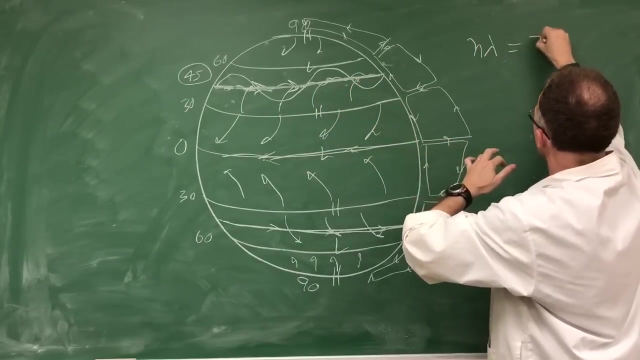 hemisphere. same thing, right, because of the movement here. so we get these jet streams moving here. but there's undulations in these jet streams. there's waves set up, okay, there's one wave, there's two waves. so typically they're set up to some quasi resonance and lambda equals to L, where L is the distance all the way around. so 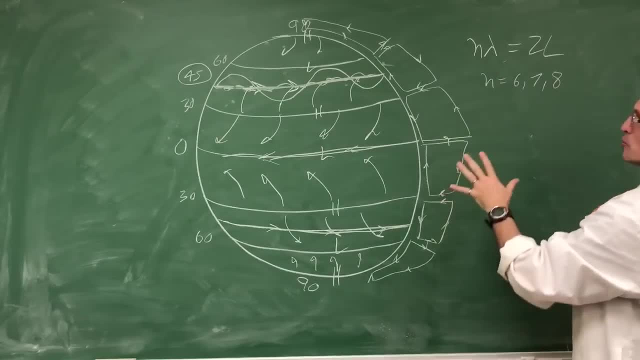 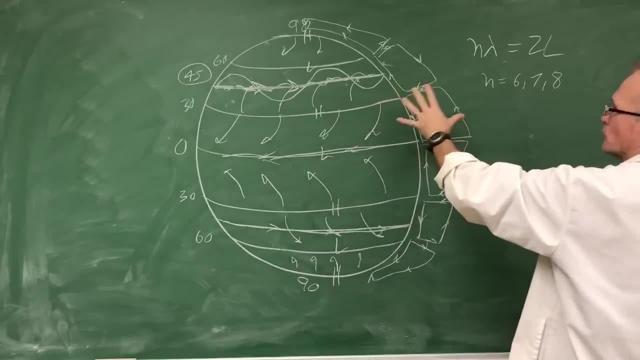 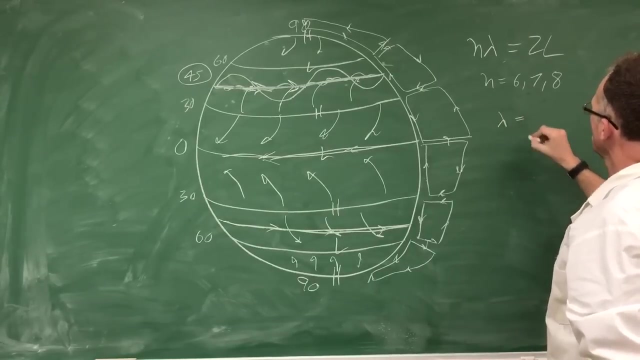 when n equals six, seven or eight, we tend to get resonances. the amplitude of the wave gets larger, it gets stuck into position. we get extreme weather events, persistent and stuck jet streams. n equals six, seven or eight. so when it's six, it's lambda equals. when it's six, we have three lambda equals L. when it's. 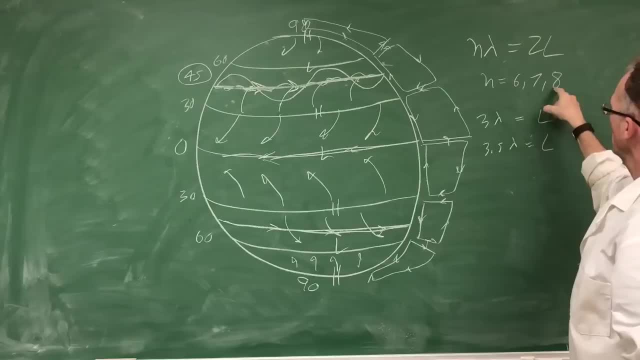 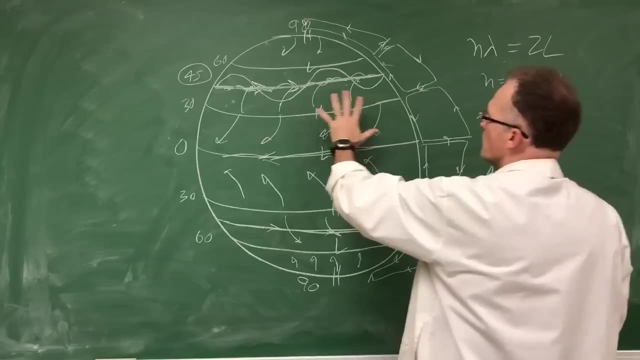 seven, we get three- point five- lambda equals L, and when it's eight we get four lambda equals L. so we get three wavelengths, three and a half or four going around. I've drawn one side of the earth. we see two wavelengths here. we'll have two on. 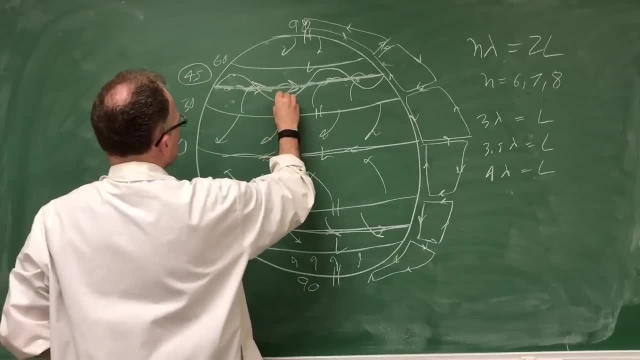 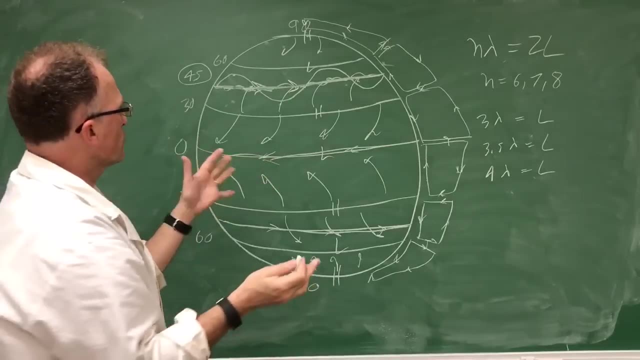 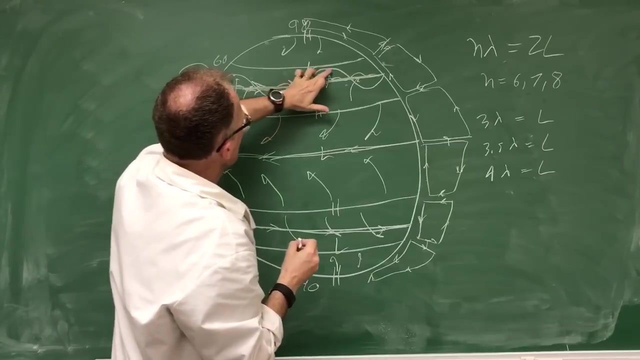 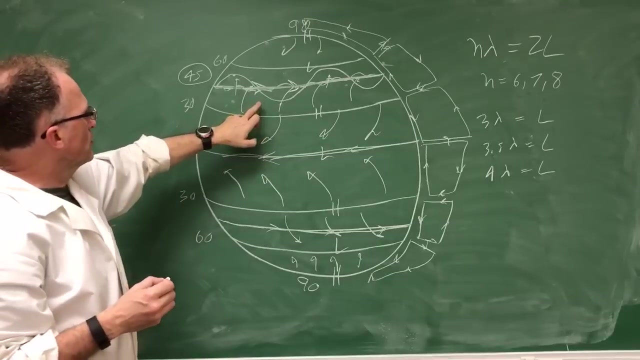 the other side. these are the rigid, these are the troughs. okay, cold, warm, hot air. warm hot air, warm, humid air from southern latitude goes up into here, here and here. so these are high temperatures underneath here, hot and humid. these are low temperatures and dry here. okay, let's say that you're sitting right here, okay, it's. 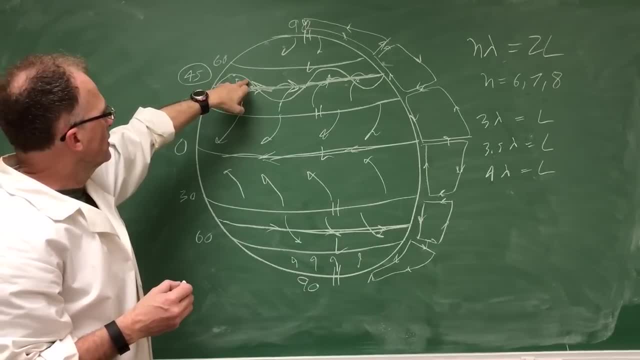 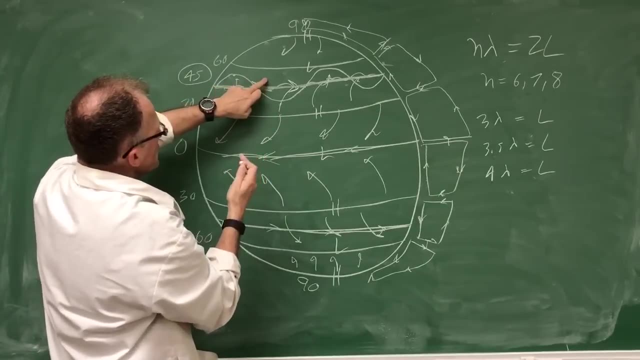 unseasonably warm for you. okay, it's warm and humid, might even be in the winter. then the jet stream shifts over, and now you're over here in the trough as this moves by your position on earth. and now it's cold and wet. okay, you're cold and 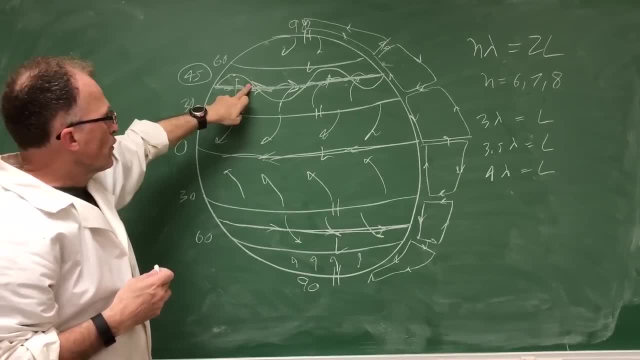 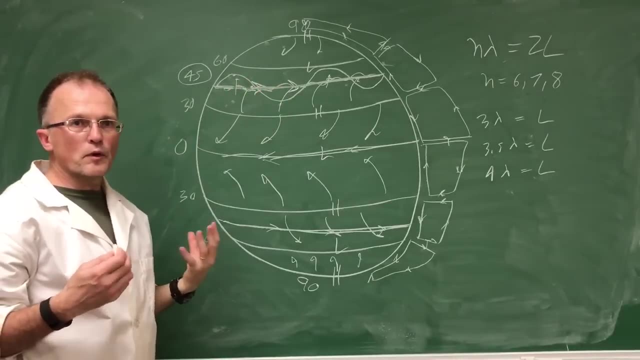 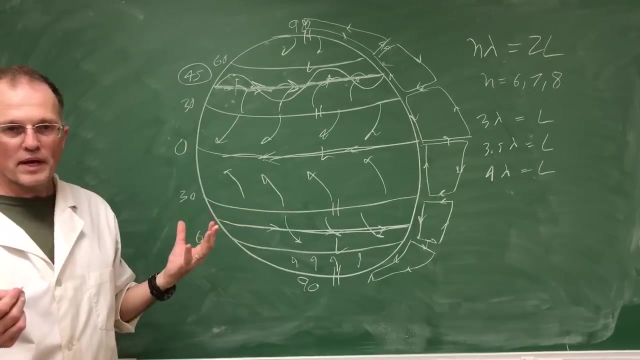 very cold and snowy, depending on how far north you are, for you know how you're know three, four days a week, and then if the jet stream shifts again, you go back. so we're getting this weather welding or weather weirding very rapid changes in temperature in a given location. so, needless to say, this has a tremendous impact on infrastructure right. imagine rail or bridges. anything metal is going to expand and contract with the temperatures. we're going to have roadways opening up like it freezes. water goes into cracks, freezes, pushes the cracks bigger. then the water thaws, percolates down deeper in the ground. 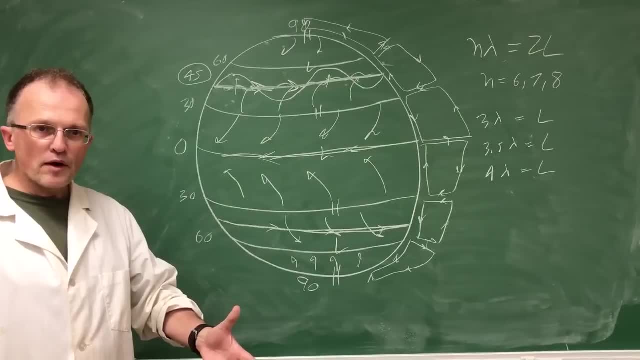 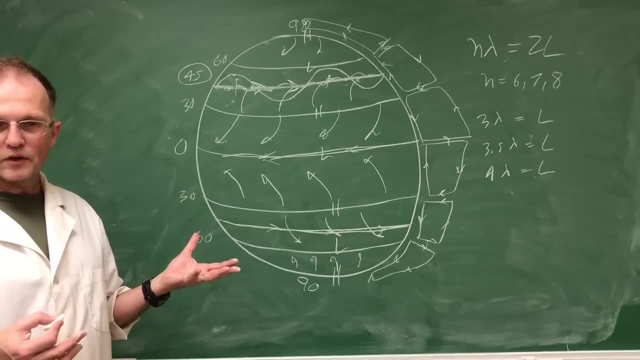 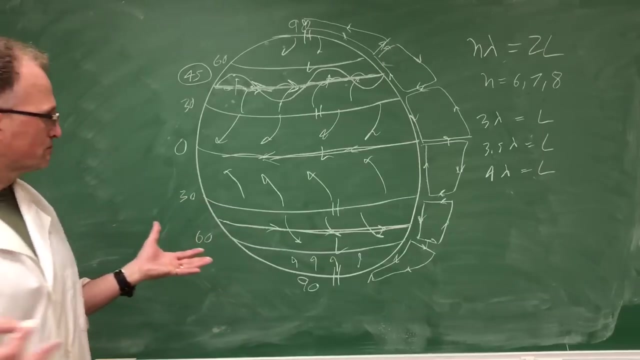 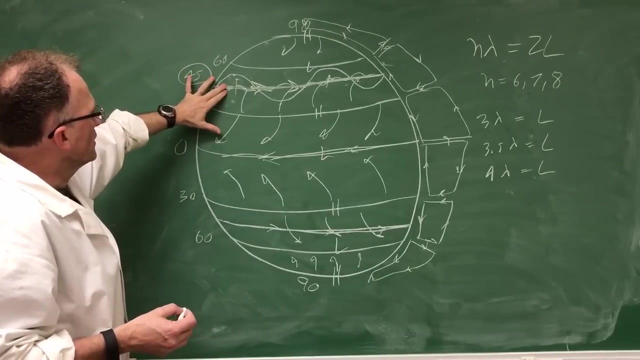 next time it freezes, the water pushes the crack open more and more and more, and so these swings of temperature, especially above and below zero, are catastrophic to infrastructure: bridges, roads, rail buildings, foundations, you name it everything, but we're just not doing anything about it. okay, so what happened now is that the Arctic, the sea, ice area, 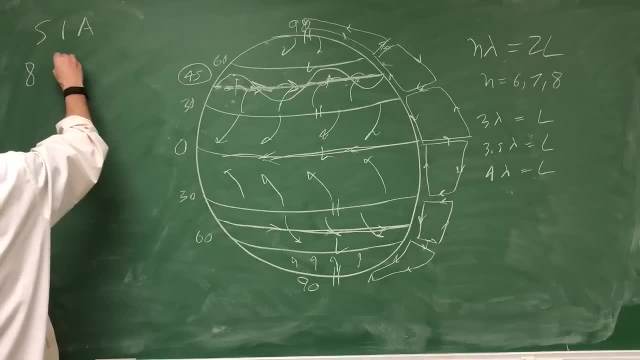 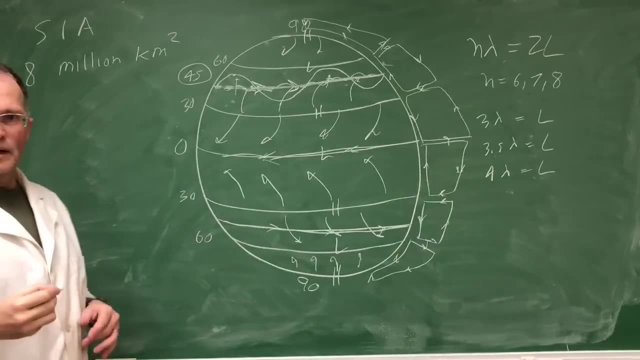 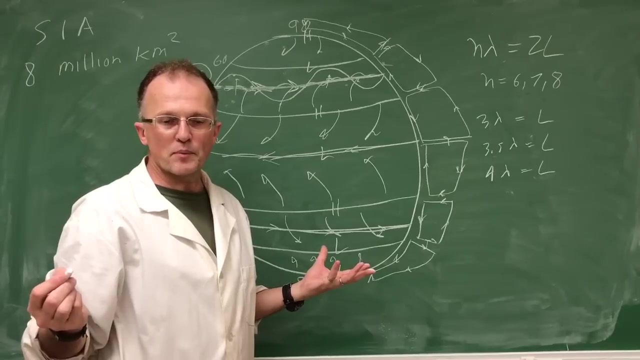 sea ice area used to be about 8 million square kilometers. okay, I'm reading. I'm rereading Peter Wadham's book a farewell to ice, highly recommended. if you haven't got a copy, pick up a copy and read it. you can read Peter Wadham's book a farewell to ice, highly recommended. if you haven't got a copy, pick up a copy or read it one by one. 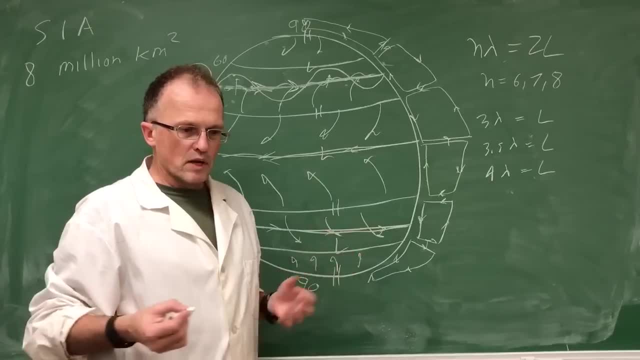 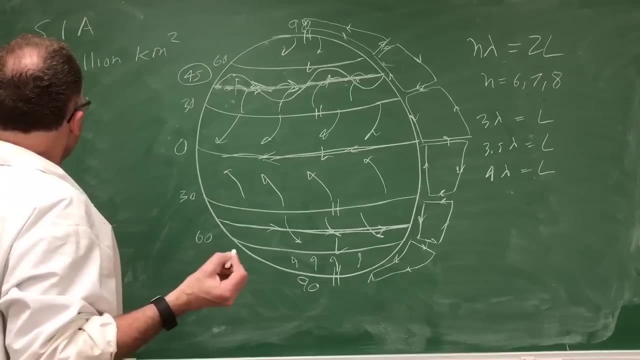 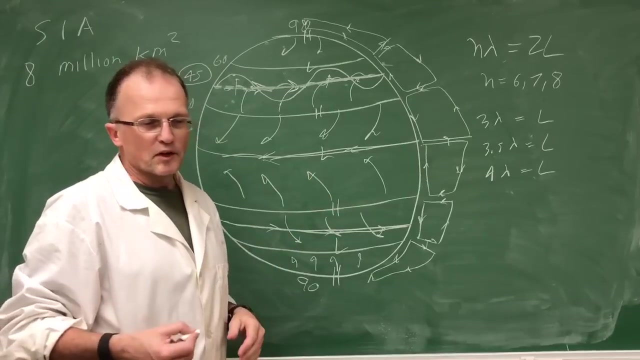 at the library, demand your librarian, get one. um, you know, get a book. even better, buy the book. you know peter can give me a cut. yeah, um, so i, i am the first person that he um, thanks, you know, in the acknowledgments for the book. but, you know, maybe that's just because i'm i'm a beckwith b. 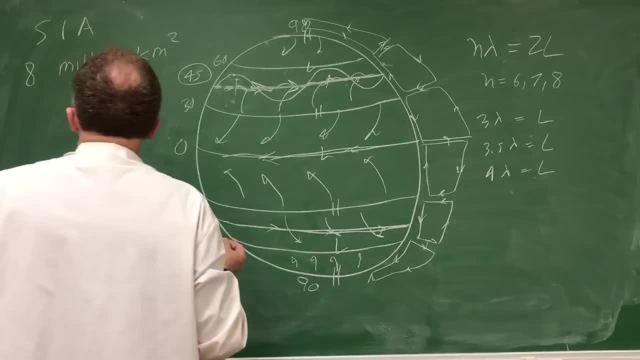 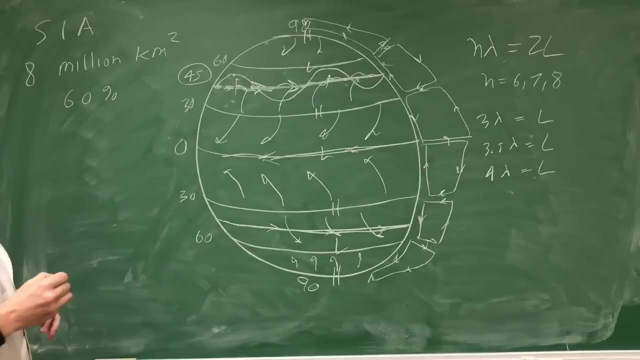 right, so maybe, maybe not. i did help them a lot actually. okay, this is what the sea ice area used to be. it reflected 60 of the light roughly on average. you know fresh snow on it, 90, a lot of melt ponds and melt areas- less than 60. you know about 60. okay, it's under 4 million now, in fact. 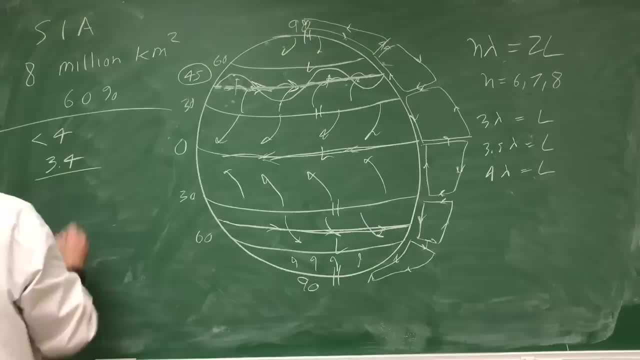 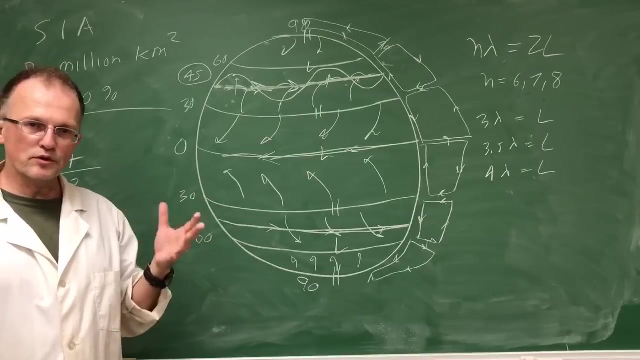 it reached 3.4 or something. you know 3.4, 3.2 or something. okay, you can look at the earth. apollo 8 was the first picture. you know, the astronauts were orbiting the moon and as they're orbiting the moon, the earth had disappeared. and then the earth comes up, earth rise when they see 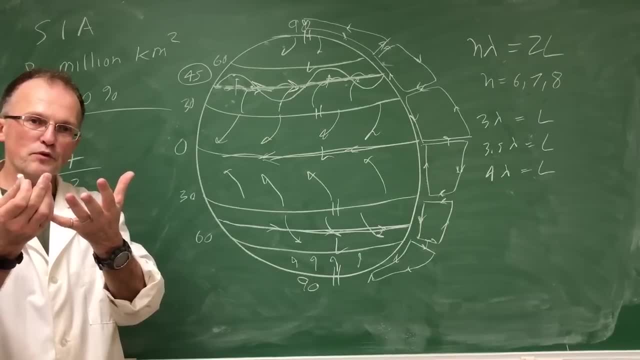 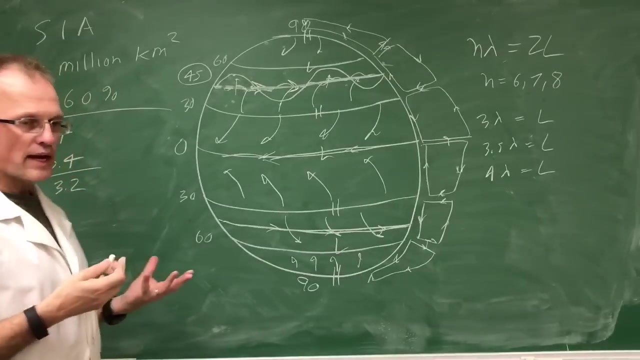 the earth. you know it's a nice blue marble, you know, just beautiful. give it gives a real, um different view on our planet. if you, if everybody, could see that, maybe we treat the planet a bit better. but there were white, two white caps on the planet. okay, the same view now. 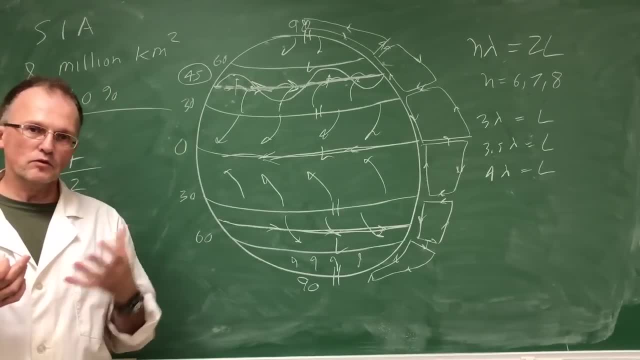 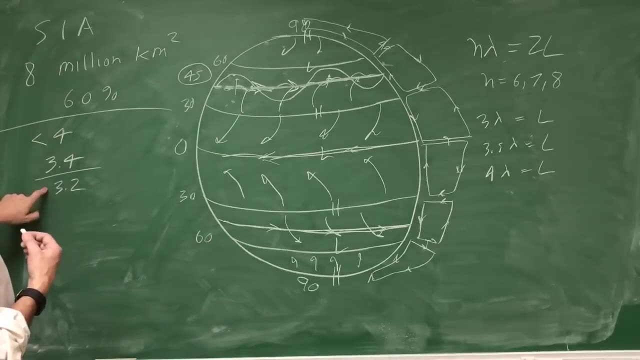 during the summer in the arctic. it's not a white, it doesn't look white so much, it's bluish on the surface. blue ocean: we're getting, we're heading there rapidly, okay, so 3.2. so the area is down and the water around reflects only 10% of the light, so you can obviously see. 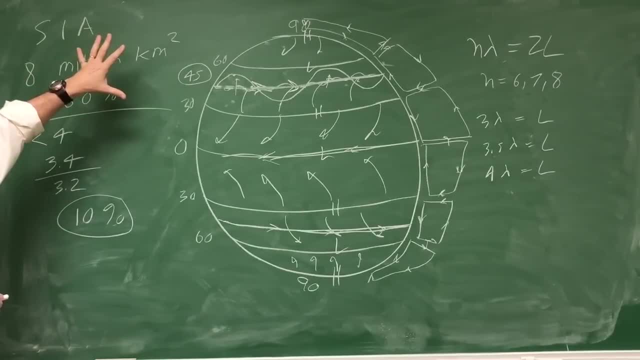 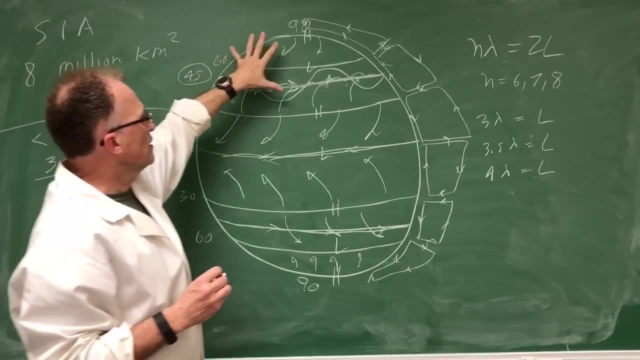 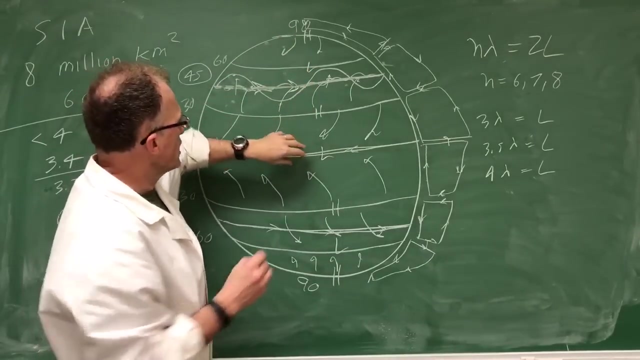 that during the summer, the sun shining on the Arctic 24 hours a day, it's being absorbed by that really dark ocean. it's causing heating. that rapid heating is causing the temperature to rise here a lot more quickly than the equator. okay, so the temperature difference, if this is rising a lot of this isn't changing that. 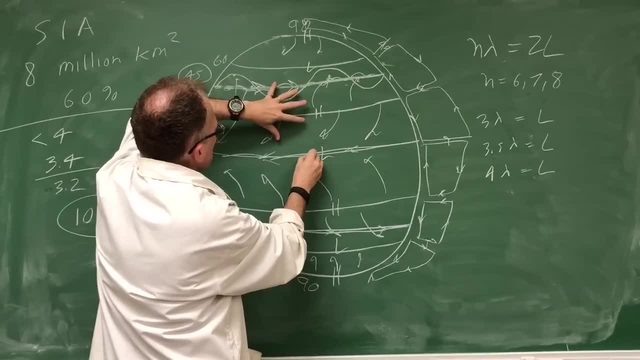 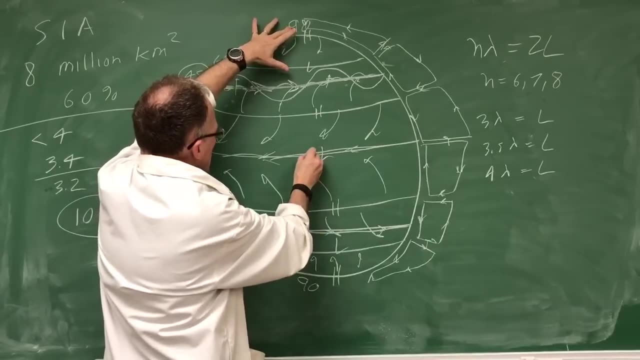 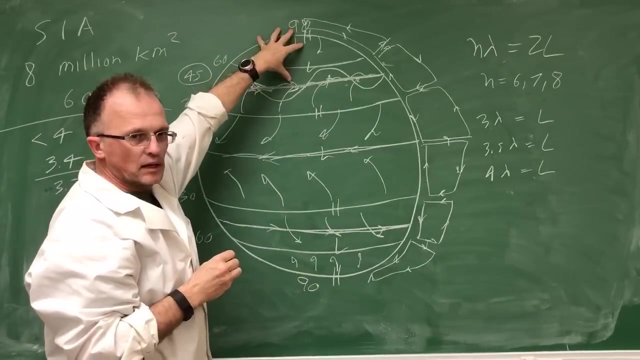 much. this temperature difference is decreasing, okay, not so much in Antarctica, right in the southern hemisphere, okay, although we're seeing changes in the sea ice around Antarctica too. but we're getting this tremendous heating, and as we get heating, then we're getting released. the land around the Arctic Ocean has a lot of permafrost. it's. 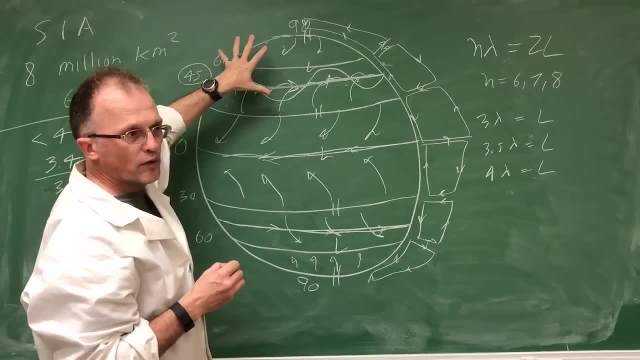 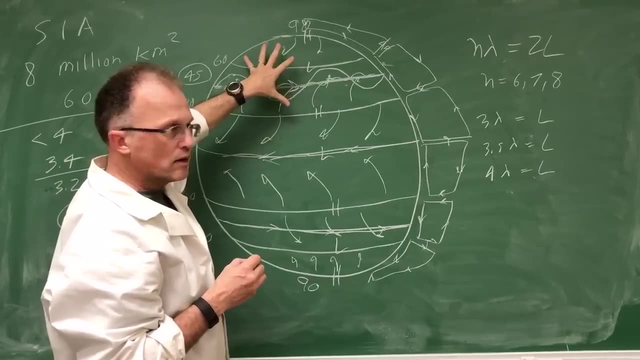 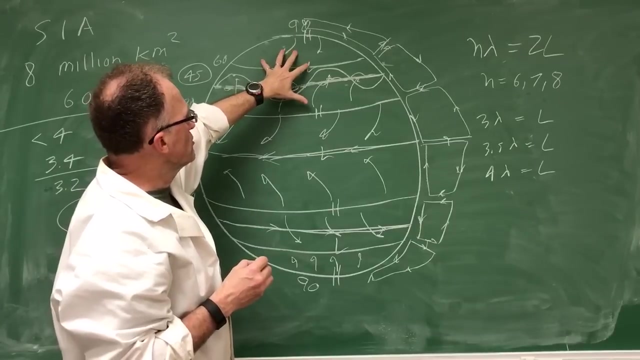 releasing carbon dioxide and methane, depending on whether there's oxygen present near the surface or whether it's underneath the water or a marsh, and then it's more methane. so we're getting those things released which are adding to the mass of heating, and we've seen regions up in the high Arctic 30 degrees Celsius. 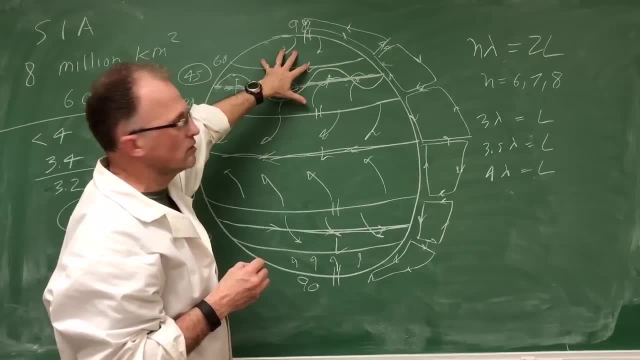 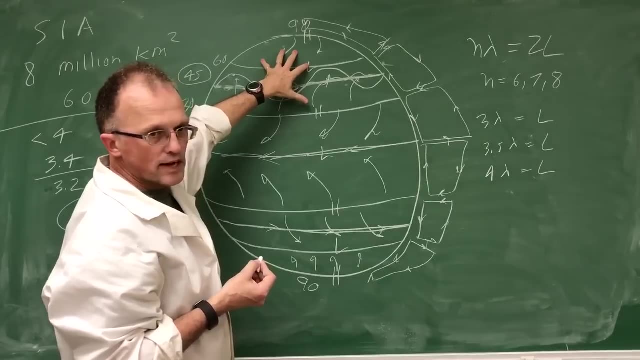 warmer than normal for long periods of time on end and the sea ice is setting up. it didn't form properly this year. it's super thin and it's ready to to go. we're getting large export out of the Fram Strait and so on, so you know we're. 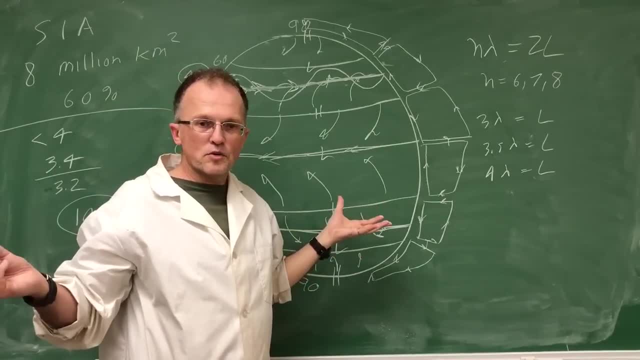 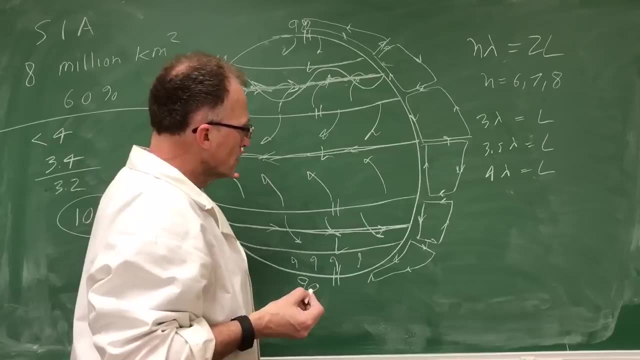 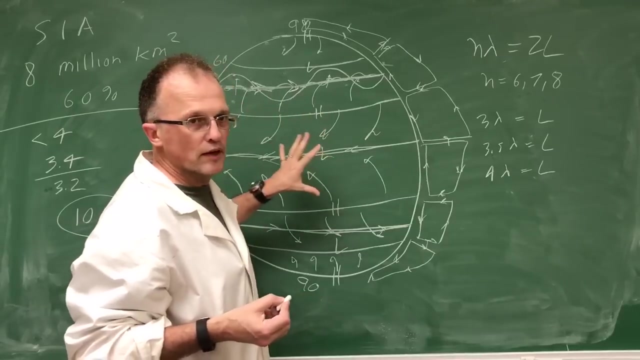 everything is changing we. this is an emergency situation like there's no question scientifically. it's an emergency situation. we need to take action. we need to be aware of it because it's going to affect everything on the planet, as you can see. it's going to affect wind circulation, ocean currents. 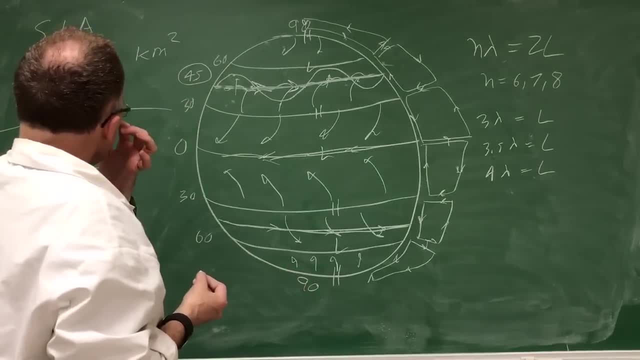 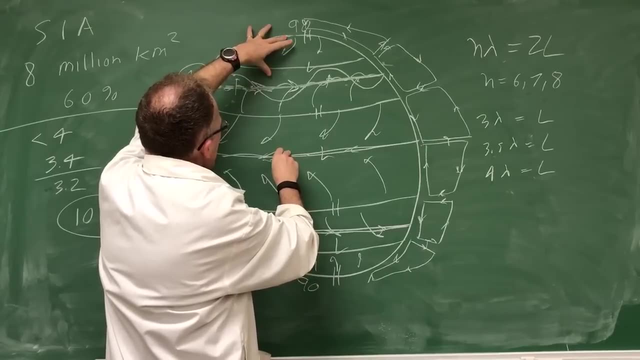 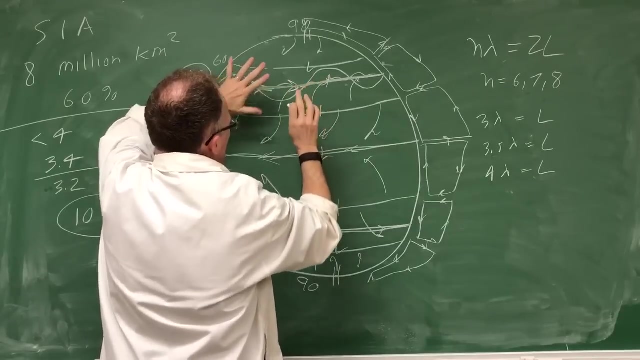 it's already doing that. so what happens when the temperature, the reason why the jet streams are formed, is because this is a high here and this is a low here, and you get this movement of air and you go up high and you're above the boundary layer of the 1.5 kilometers. 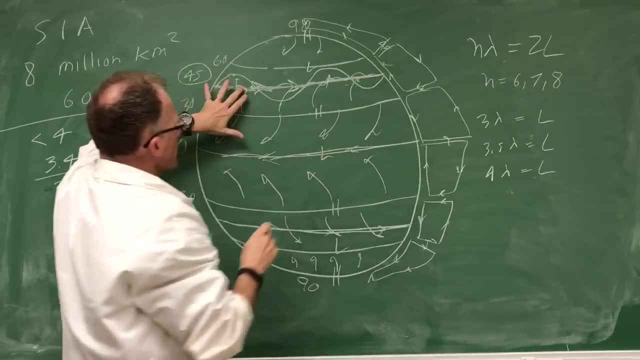 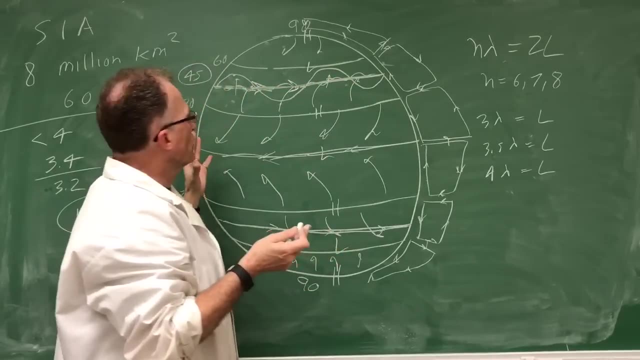 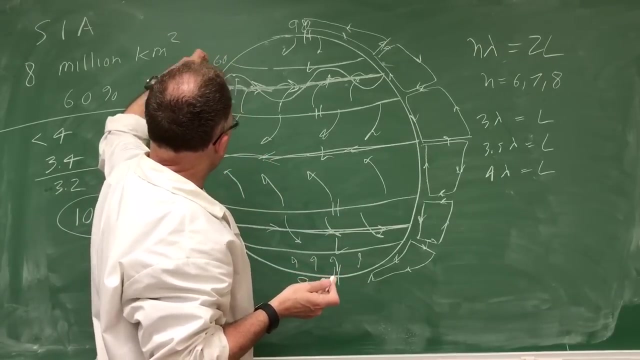 you get geostrophic flow and you get this air movement and there's perturbations to this, this direct zonal flow, by a number of factors. that's not a stable state. topography, like mountain ranges, affect things. it can't go through the mountain range. it has to go up above it or below it and that leads to pegging it. 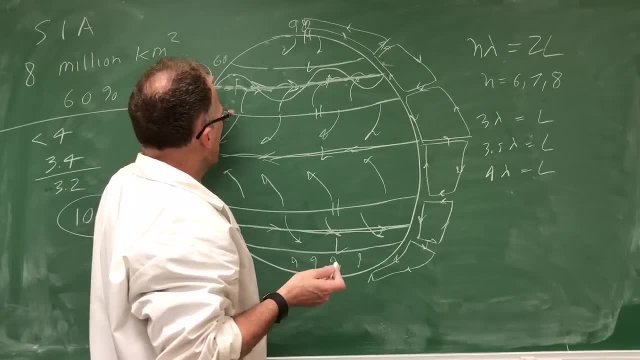 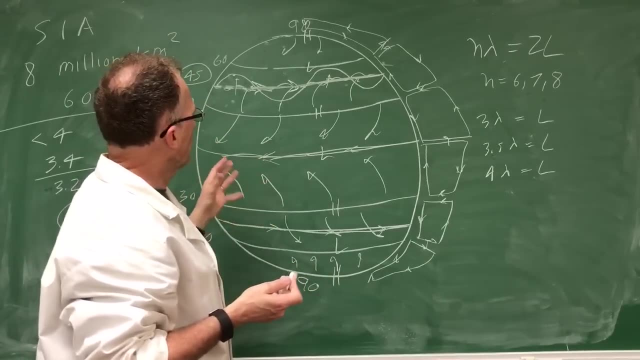 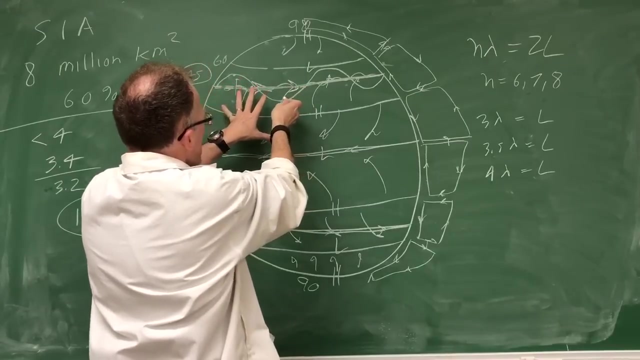 at certain locations on the earth there's also a lot of contrast between um the land and the ocean. for example, in the summer the land is a lot hotter, the ocean is a lot colder, so that thermal gradient causes the high and low pressures to be offset in the direction, depending on the geometry of the water body, and that causes perturbation. now, when 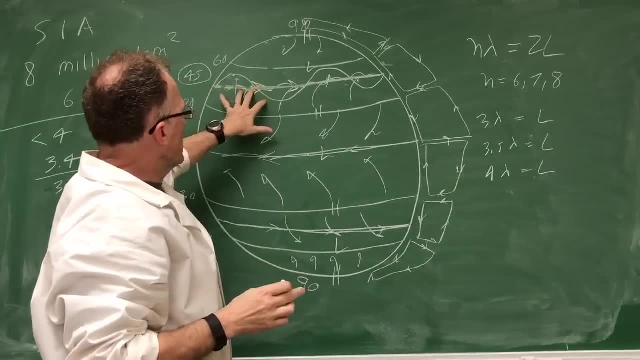 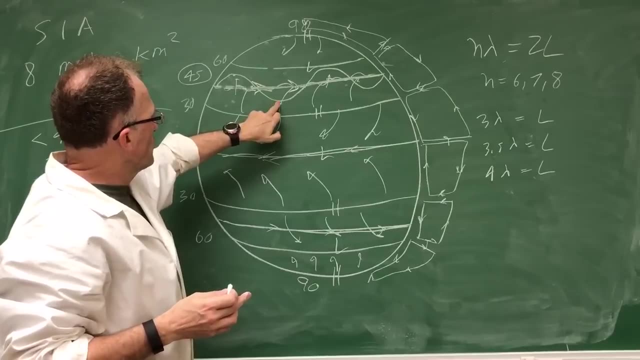 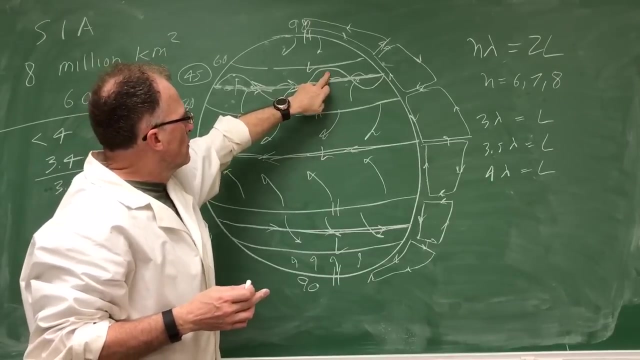 we get into this particular pattern, then we get amplification of these waves and it can get stuck. uh, think of 2010. the. the trough was over Pakistan, stayed there for 30 days, flooded out three-quarters of the country. the crest was over Russia, over 30 degrees Celsius. for 35 days or so, they lost 40. 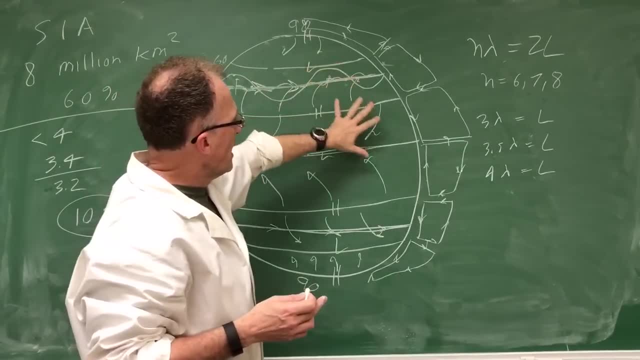 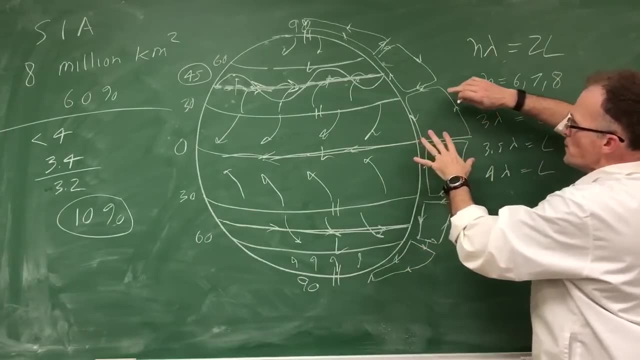 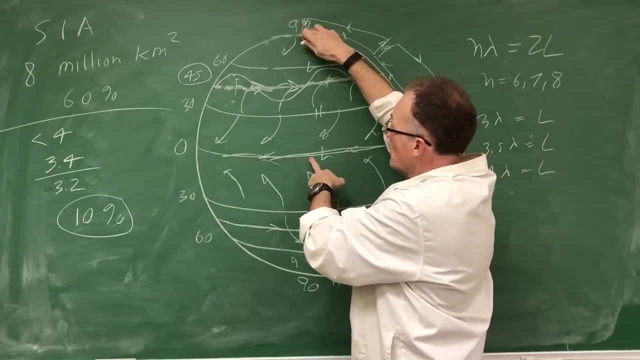 percent of their grain crop. this has huge implications. what happens to the Hadley cell? okay, so as we get warming, as as the temperature gradient, first of all, let's say this is now the same temperature as this, just a thought experiment. it will always be slightly colder, okay, but not. 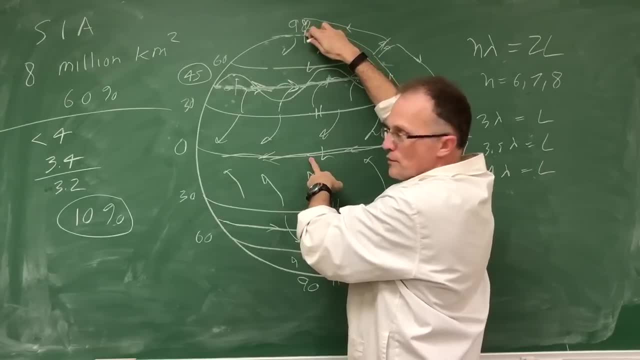 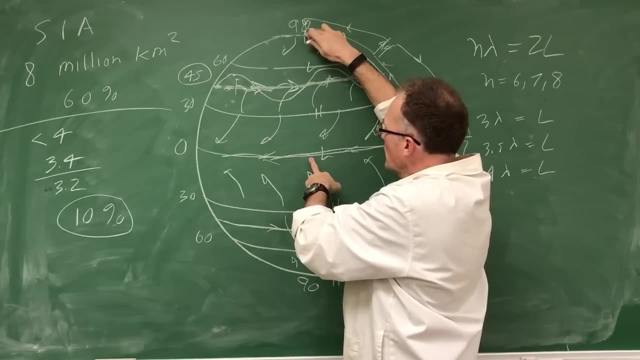 much colder if there's enough heat transfer or if there's enough absorption. in the summers, everything is so dark, no ice and snow in the entire Arctic- okay, and then there's the jets. don't forget the way where the jets are. this is bringing heat north and this is bringing 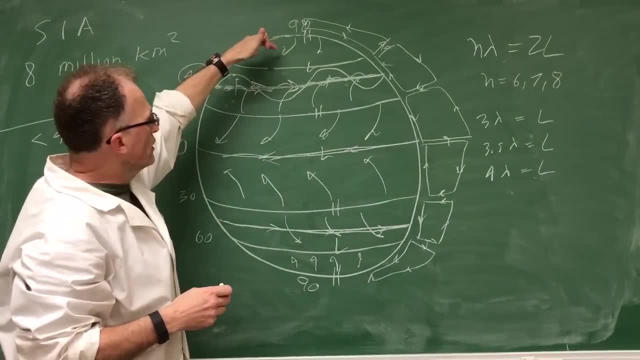 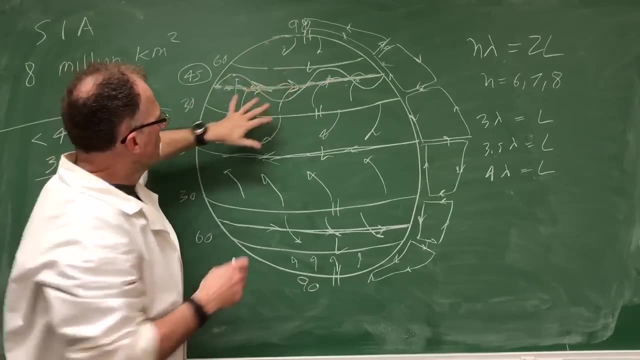 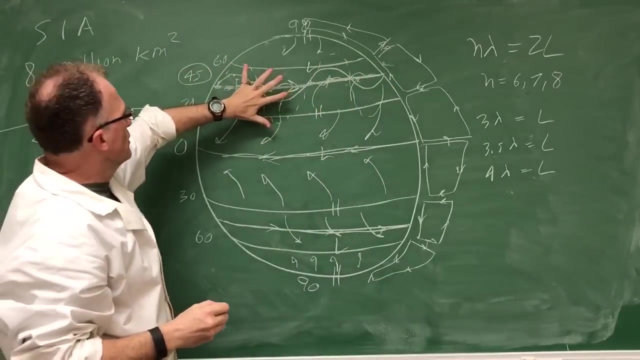 cold South. bringing cold South is taking away cold from the Arctic. it's replaced by heat. okay. so the wavier the jet streams, the more heat transfer there is as they become much wavier. okay, they pretty much equalize temperature. in the northern hemisphere also, we've seen periods of time where 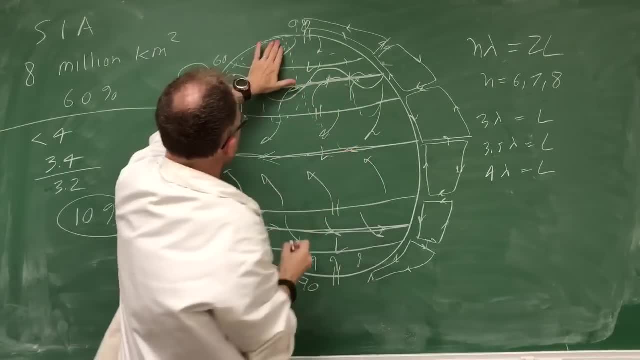 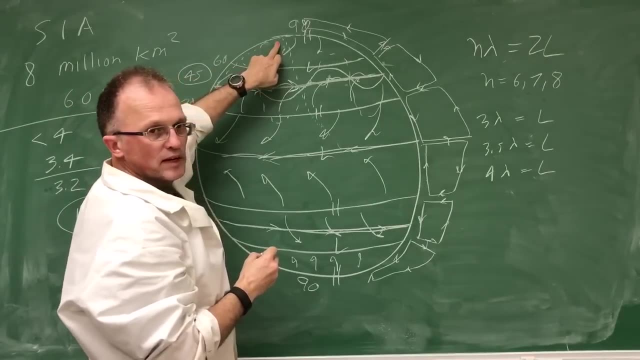 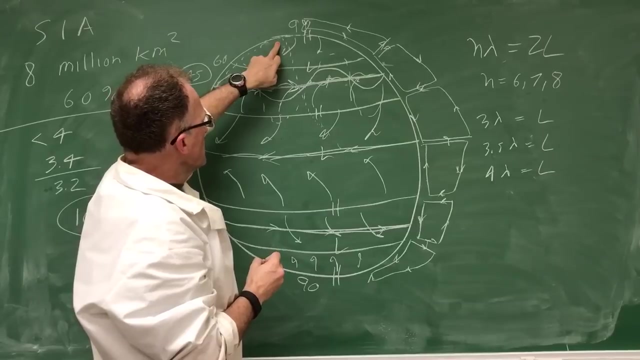 where they become basically they, they. we've seen periods of time where the, where the bridge of the jet stream has gone right into the Arctic, bringing the temperature above zero in complete darkness in the middle of the winter. you've seen that multiple days. okay, that's happened. we've also 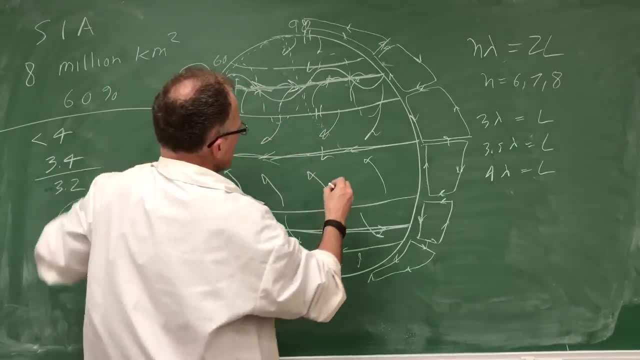 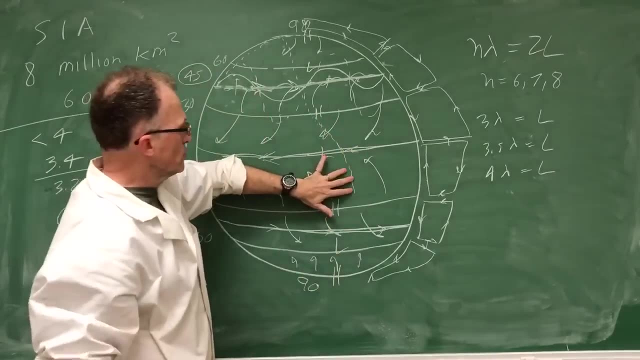 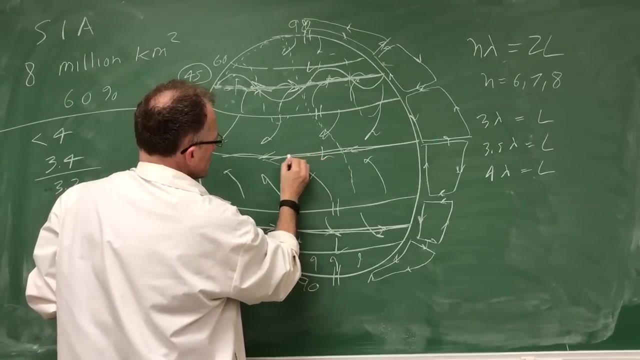 seen areas, as I pointed out in a video um about nine, ten months ago, that the jet stream was going so far South that it actually crossed the equator joining with the jet streams in the southern hemisphere. there's monsoonal flow over the equator from time to time, but that's pretty. 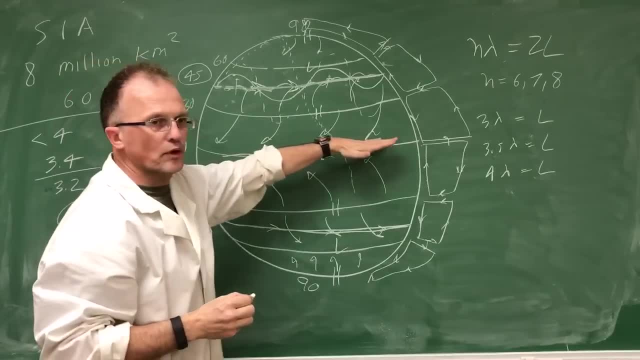 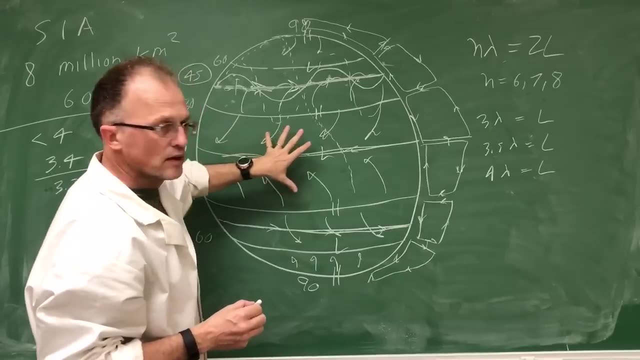 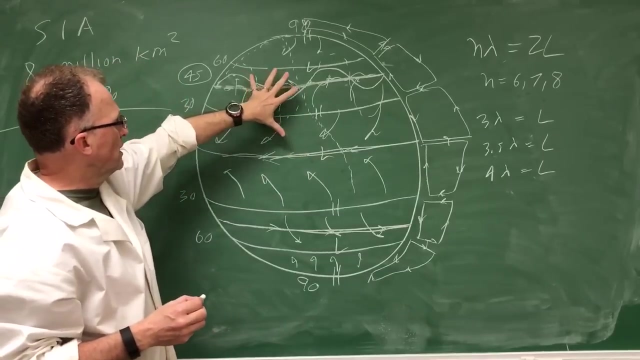 much parallel or at a slight angle to the equator. to the equator, when it's coming across a normal incident in multiple places and strength, then it's breaching and it's causing more of a mixing between the the two hemispheres. okay, so this is explaining the extreme weather in the northern. 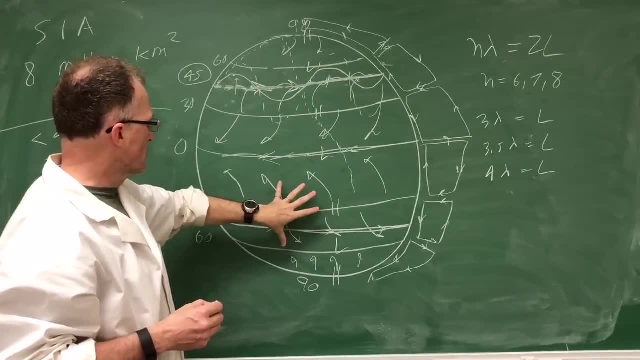 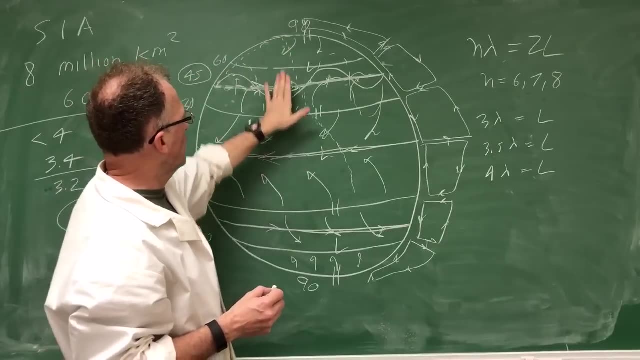 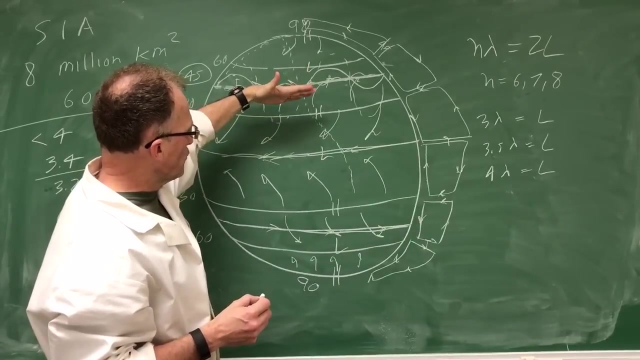 hemisphere, southern hemisphere, doesn't get away scot-free right because, look, this is hot, this is cold heat, and go to equalize the temperature. why is this hot? because it because the sun is is in it's, either if it's over here or over here throughout the year. it's oscillating about this position. 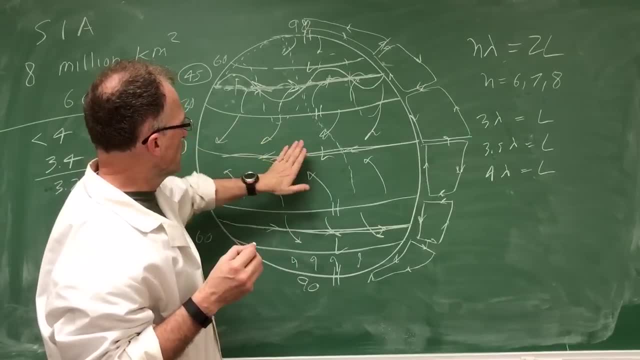 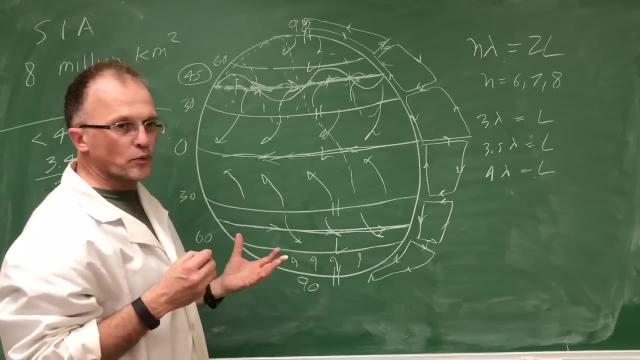 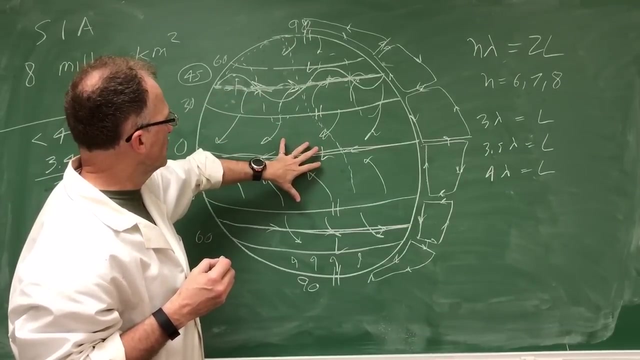 the sun is going directly through the atmosphere, which appears thinner. if you're at a grazing angle, the atmosphere is sicker um. so the energy intensity, the watts per square meter um, is much greater here than here. this is always 12 hours of light, 12 hours of day, of night. you know this will. 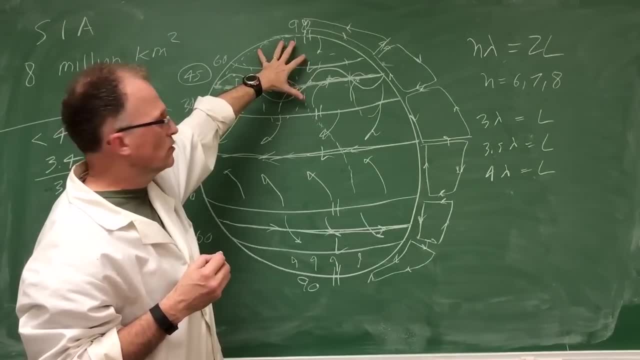 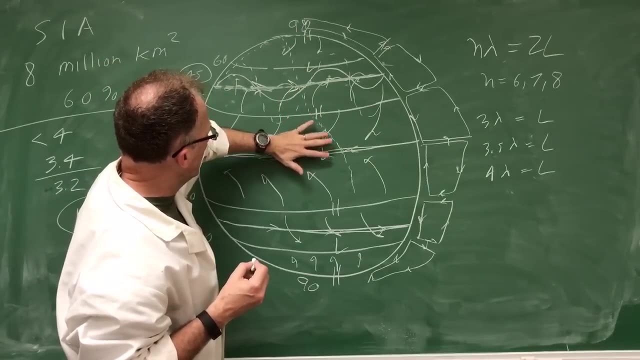 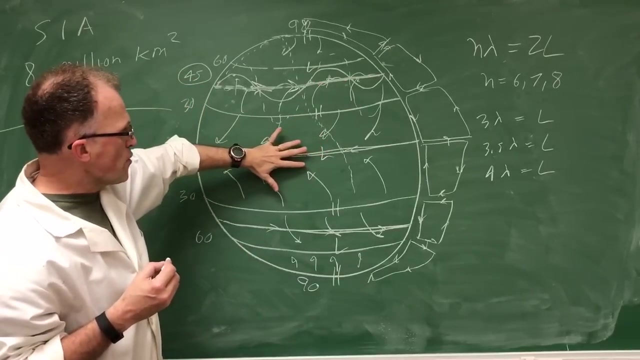 be complete seasons of darkness, complete seasons of lightness. okay, so all of these factors? this is colder, so less heat will go from the equator to the pole here, making the jet streams way bigger here. where does that heat go? you can evaporate more water right at the equator. it. can increase the intensity of the of the water and then the temperature of the water will go up. in fact, for every degree celsius increase in a region, you get seven percent more water evaporation, seven percent more water vapor in the atmosphere, so that heat, water heat- is going to the southern. 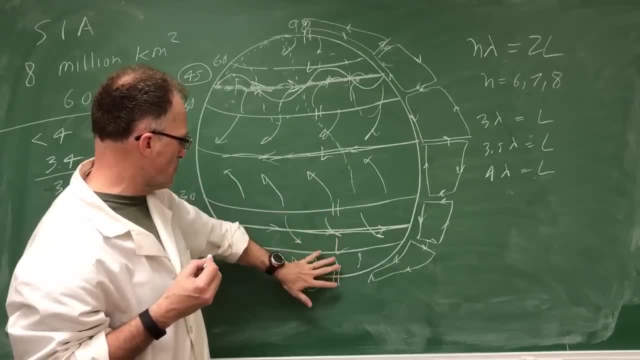 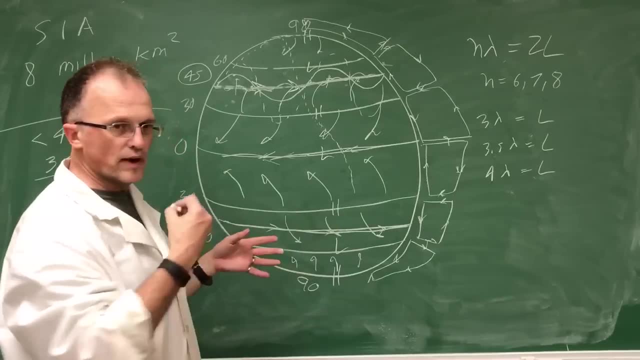 hemisphere. it's coming down as far as australia because there's a large temperature gradient. antarctica is still cold, so it creates a very, very strong southern annular mode. the winds around antarctica have been larger now. up to recently it was pulling the ice away from. 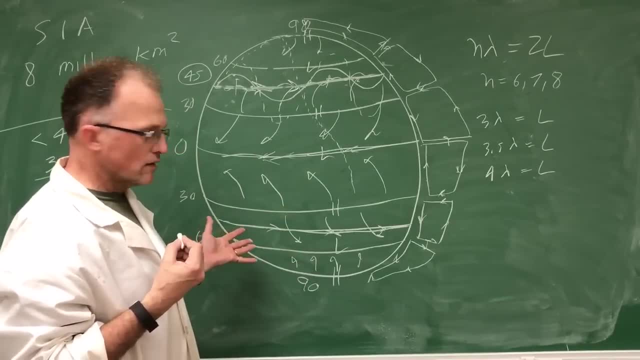 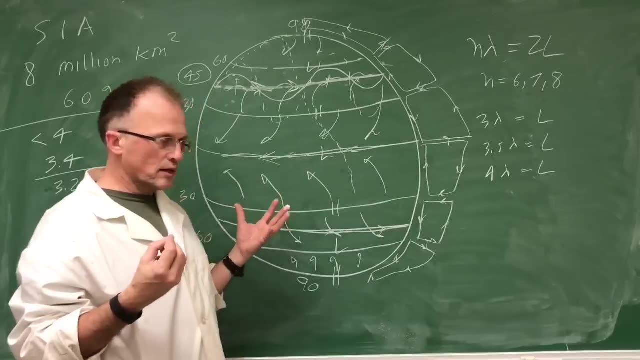 antarctica making record high levels in sea ice, and then, a couple years later, we're at record lows. so there's lots of oscillations. there's lots of things. this is not a. this is a, you know. i'm trying to get to the root of the things that are important.